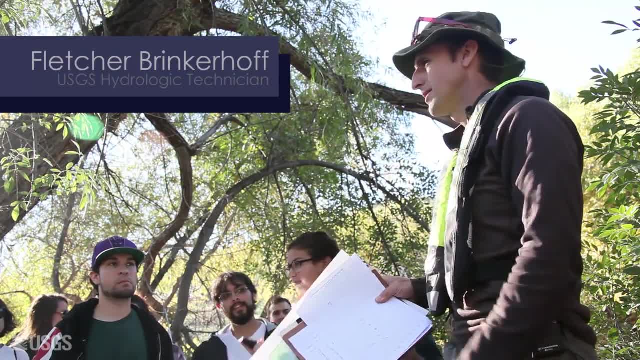 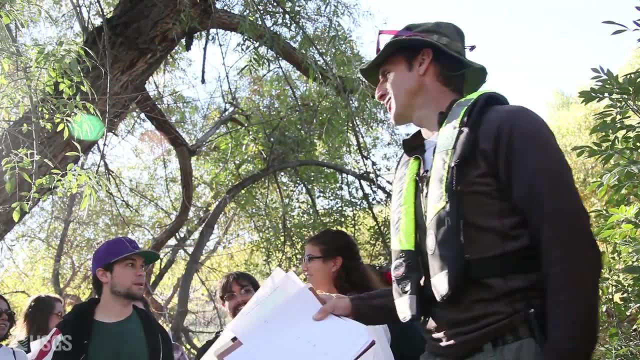 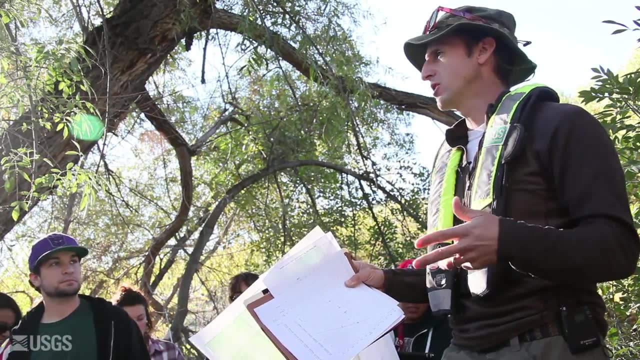 and where? Minnesota, Ohio. How do you guys like our rivers? Oh, they're there, They're just dry, And so a lot of the channels that we deal with are sand, and so they're very. they're variable, They change a lot with every flow event. They're not as stable as you would expect if it was. 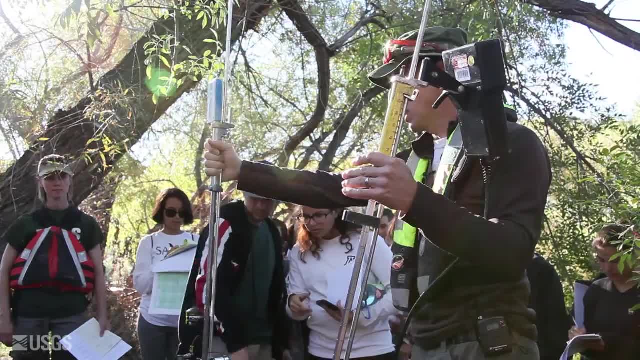 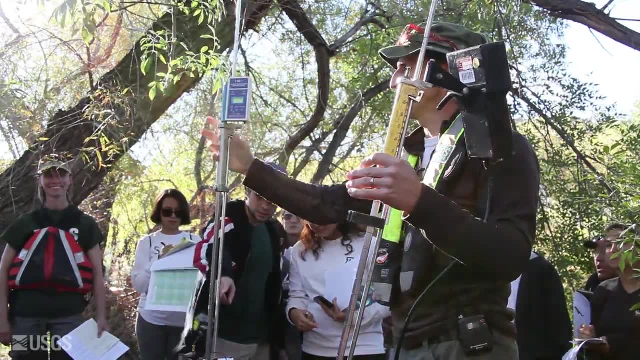 like cobble, gravel, boulders and stuff like that. Today we're using this small guy. It's a pygmy On the top. here we have this fancy device and it counts how many times this revolves. Inside here there's a little magnet. It goes past a little closure. It reads how: 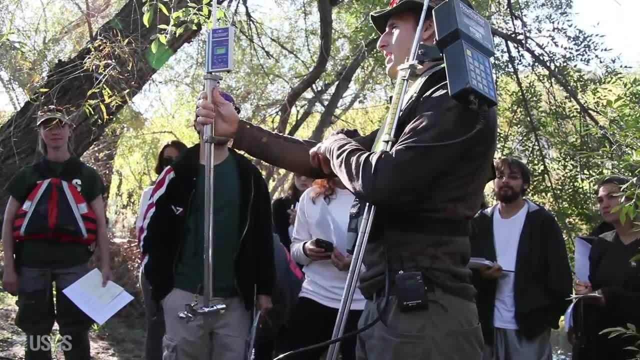 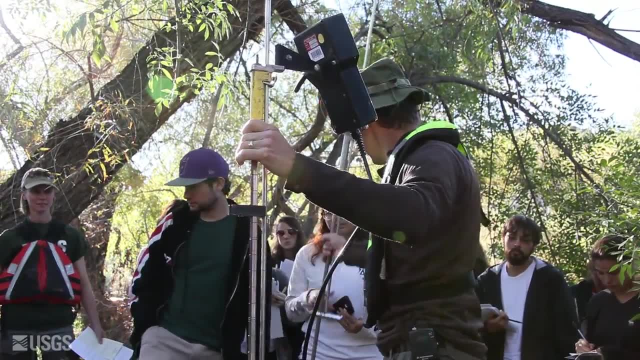 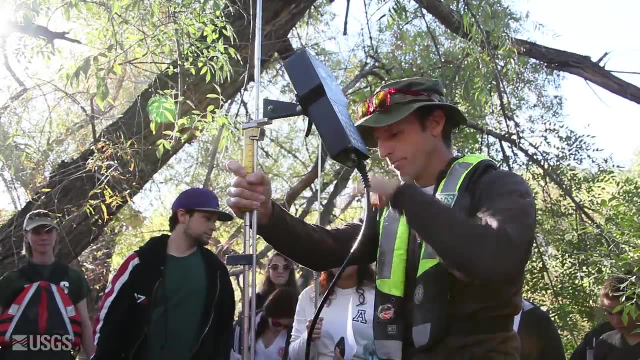 many times. it spins in a 40-second period of time and it displays it up here. Here. this is an acoustic measurement meter. There you go, Thank you. It has a fancy calculator on top. That's all it is. It's a computer calculator. What it does is it reads the flow as it comes past. 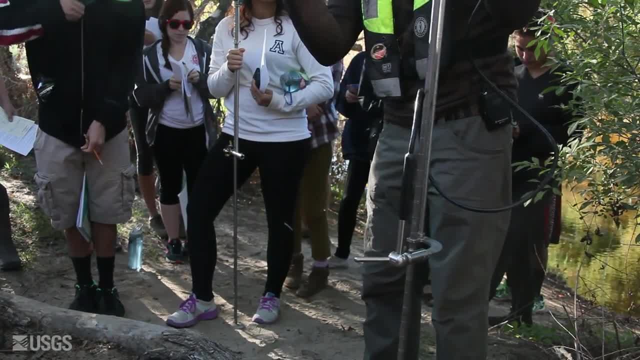 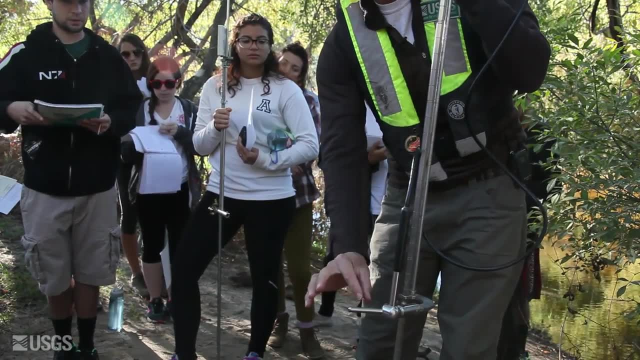 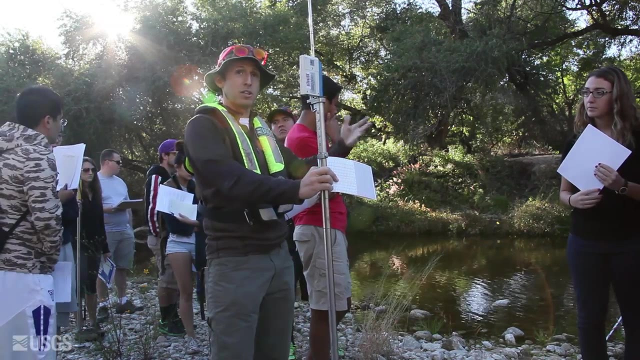 this meter. It uses the Doppler effect, if you're familiar with that, And just so you guys know, it's reading an invisible little square right about here. So do you guys understand how you compute the area? You get your widths, You get your depth, You get your area. Each one of those little 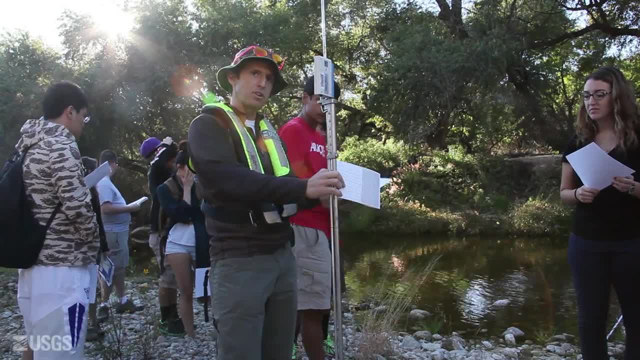 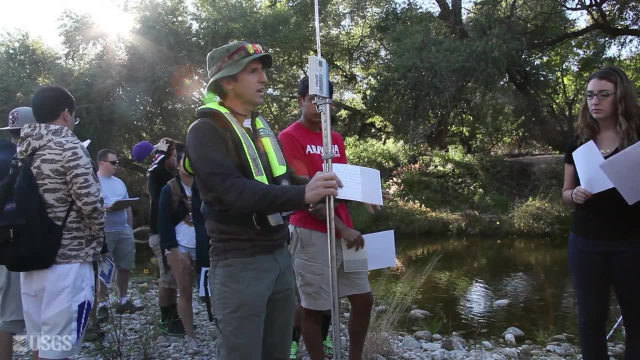 observation widths and depths is assigned a velocity for every observation, Then you can compute a discharge for every single observation. You add the total up at the end You have a total Q for the whole entire measurement. You get a mean velocity for the whole measurement. 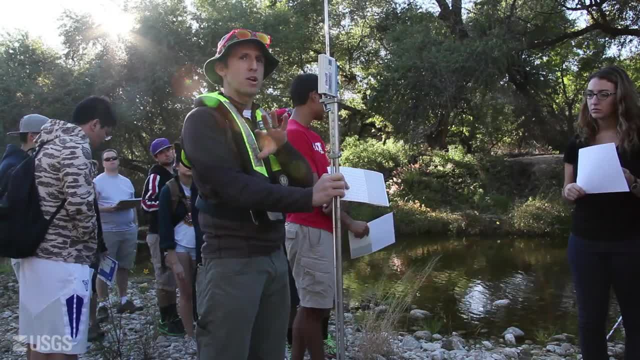 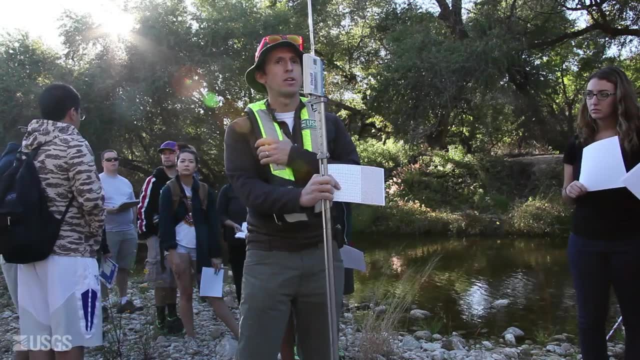 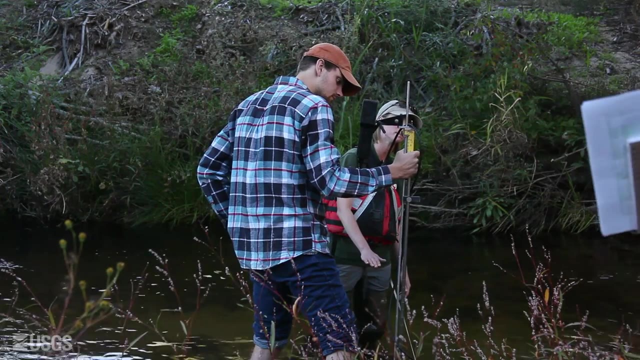 You get a total area. You kind of look to make sure the numbers rhyme and then you call it good. Any other questions? All right, Let's get in the water. Yeah, Let's go. Yeah, So at each station we're setting it to six-tenths of the depth in the water column. 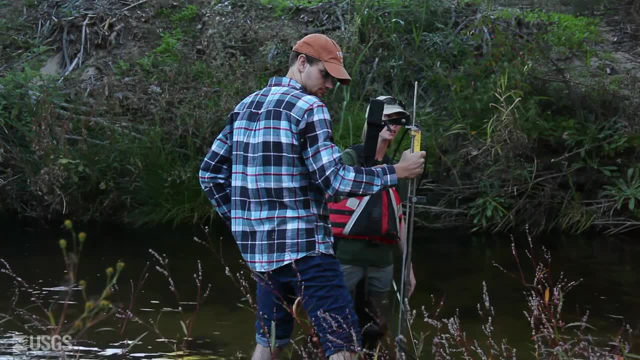 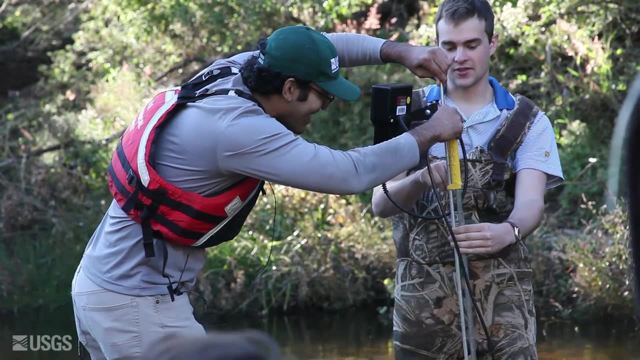 And that's the point that is representative of the average velocity at that point. Yeah, This is zero, So everything on here is a point, something now. So that's 0.5.. Oh, I thought that was 0.5, right there. 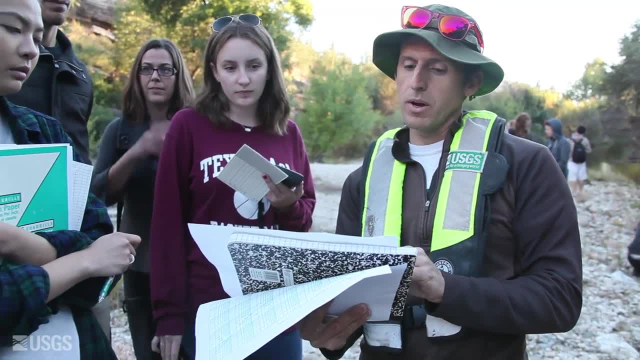 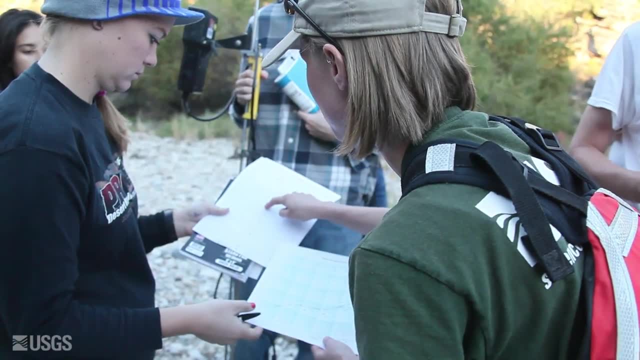 Yeah, It has been my pleasure to be collaborating with the United States Geological Survey and having this stream-gauging field trip be part of this, Thank you. Thank you for being part of our course. I'm excited because my students get to interact.